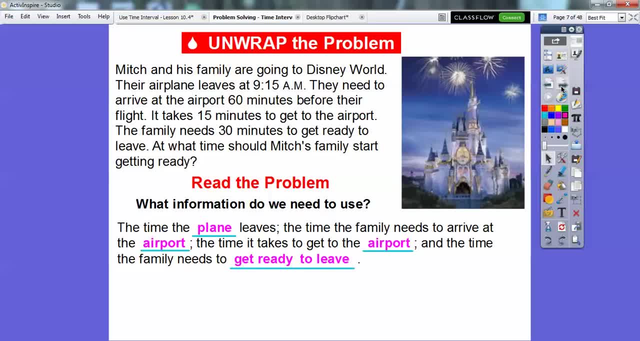 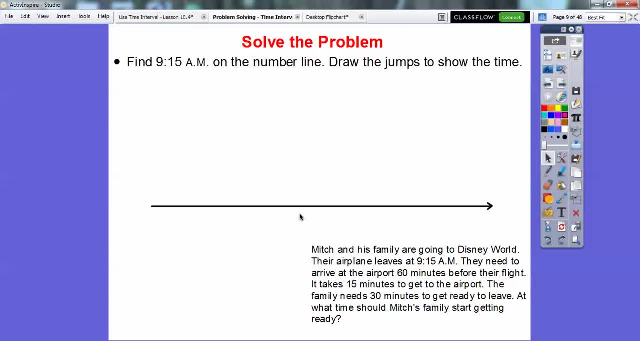 So there's lots of times that are inserted in here, So we're going to go ahead and use a number line to help answer this. So here's the problem. I shrunk it up down here and here's our number line, right here. 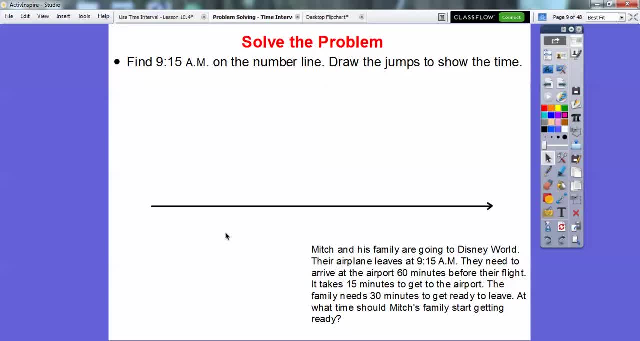 Sorry, I didn't put an arrow on this side, but that doesn't matter. We're going to start over here on this side because we're going to find 915 on the number line and then we're going to draw jumps to show. 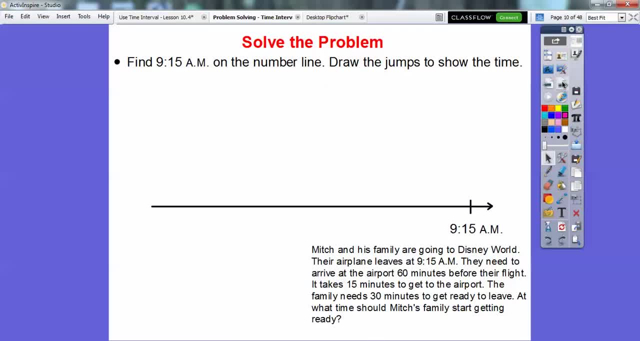 Okay, so there we are at 915, right there. Okay, so right here at 915,. and then they need to arrive at the airport 60 minutes before their flight. So let's do a count back 60 minutes. So let's do a count back 60 minutes for the time that they need to arrive at the airport, okay. 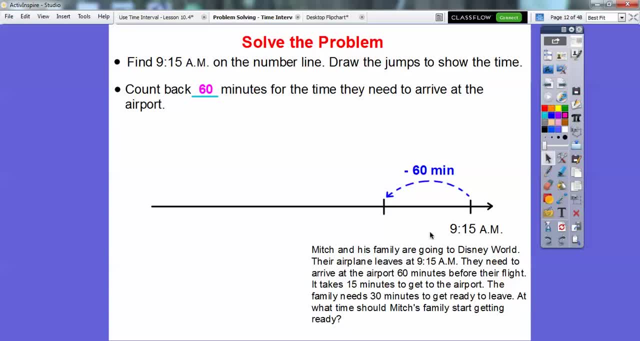 I should have highlighted that in red. I did. on the next word problem. you'll see right there. So let's go back 60 minutes. Well, 60 minutes is a full hour backwards, you guys. So if it's at 815, then we're going to have to go back to, I'm sorry, if it's at 915,. 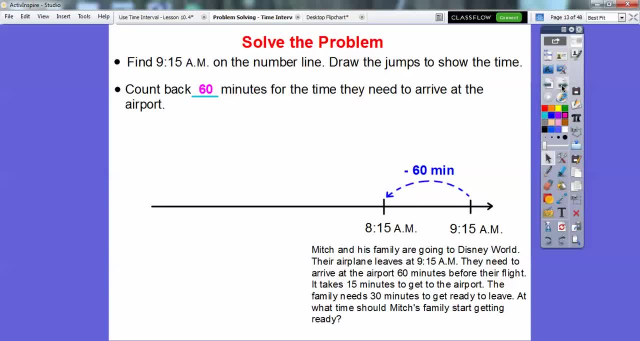 we're going to have to jump back a full hour to 815 right there, okay. And then the next part says: count back how many minutes for the time to get to the airport, okay, So we're going to go ahead and go back 15 minutes. 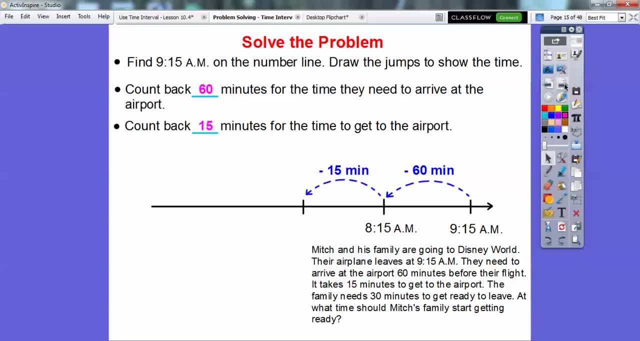 So if it's at 815 here, then take off 15 minutes and that's going to take us to 8 o'clock, right there, okay, And then we're going to count back how many minutes to get ready. Well, right here it's highlighted in red: 30 minutes to get ready. 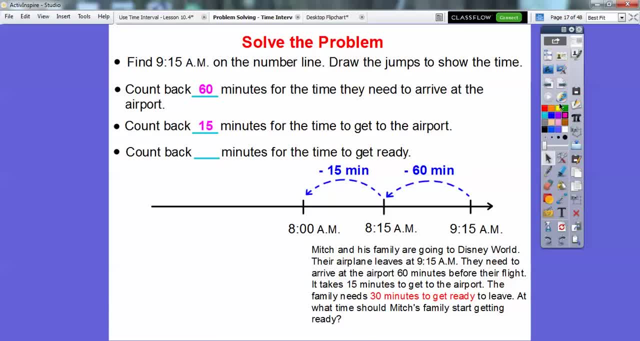 So we're going to go back 30 minutes. So 30 minutes is a half of an hour, So 30 minutes off of 8 o'clock. that's going to take us back to 60 minutes. Okay, That's going to take us to 7.30, right there. 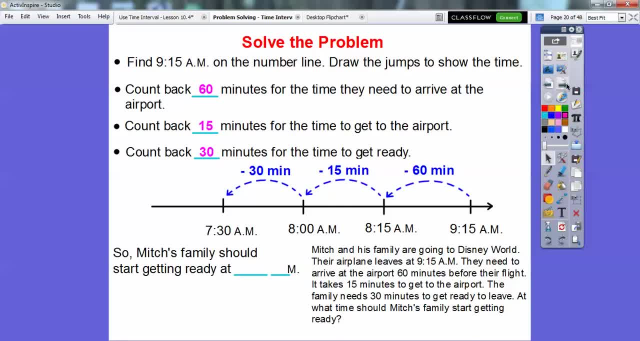 So let's answer the question. So Mitch's family should start getting ready at 7.30 am, right there? okay, Make sense, you guys? All right, Let's try another one here. So how can we check our answer? to start with, the time the family starts getting ready. 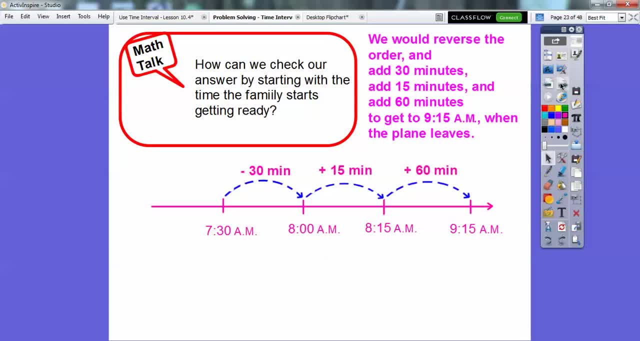 Well, what we can do is work backwards, you guys, We can go in the reverse order and add 30 minutes and add 15 minutes and then add 60 minutes. So if we started at 7.30 and added 30 minutes, whoops, that should be a plus sign right there. 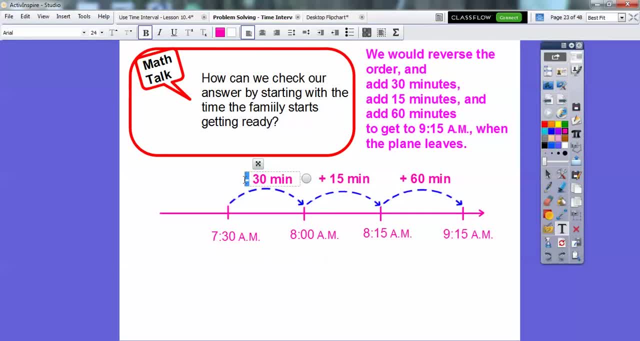 I didn't catch that. This should be a plus sign right there. Add 30 minutes. That will take us to 8 o'clock. And then add 15 minutes. It will take us to 8.15.. And then add that 60 minutes. 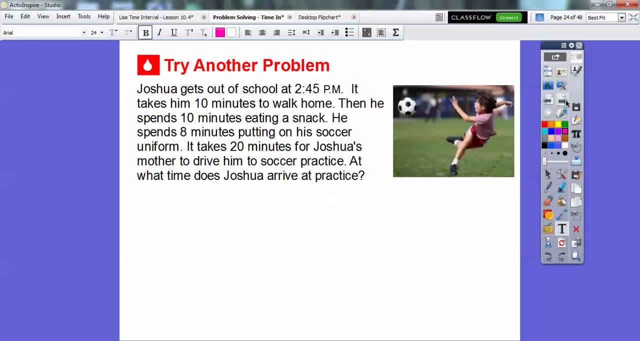 It will take us to 9.15 when the plane leaves, So we can check our answer by working backwards. Okay, Here's another one. Joshua gets out of school at 2.45 pm. It takes him 10 minutes to walk home. 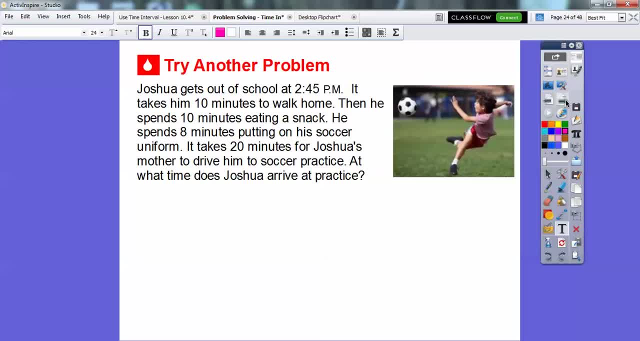 Then he spends 10 minutes eating a snack, He spends 8 minutes putting on his soccer uniform, And it takes 20 minutes for Joshua's mother to drive him to soccer practice. So at what time does Joshua arrive at soccer practice, given all that? 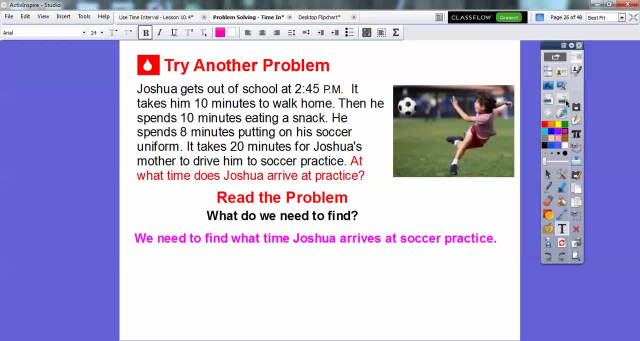 Okay, All right. So let's go ahead and read the problem. We need to find what time Joshua arrives at soccer practice, right here. That's what we need to find, All right, And what information are we going to use? Well, we're going to use the time that Joshua gets out of school. 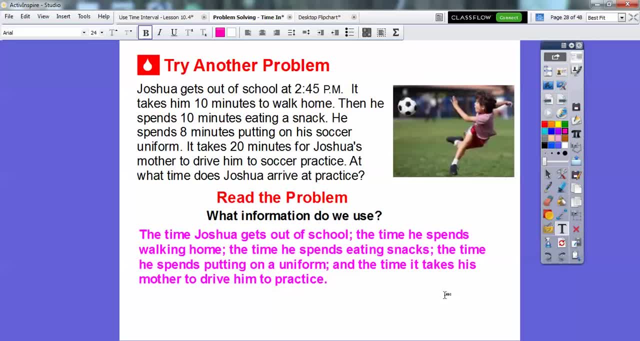 the time he spends walking home- I'm just going through this problem right here- And so the time he spends eating snacks, the time he spends putting on his uniform and finally the time it takes his mother to drive him to practice. So we're going to add all these numbers after 2.45. 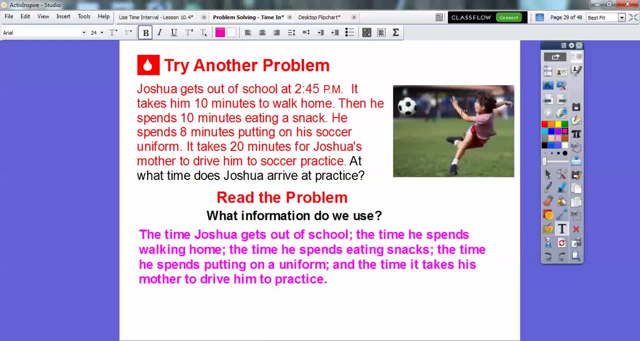 So we're going to go on the other. Now. I made this in red, you guys and I didn't like that, So I just kept it in black. Normally, I like to highlight the information that we're dealing with in red. 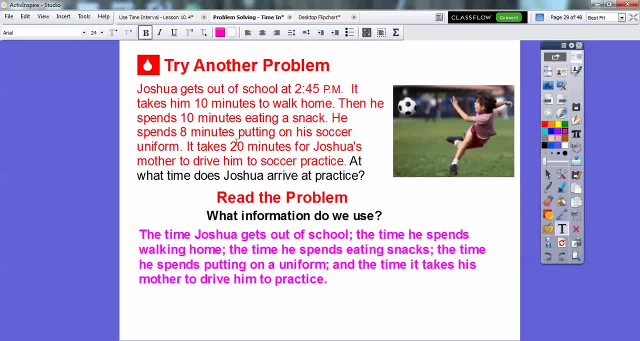 But if you look at that, that just looks kind of unpleasing to the eye. So I just left that there. So how are we going to use this information? Well, we're going to use a number line to find the answer. 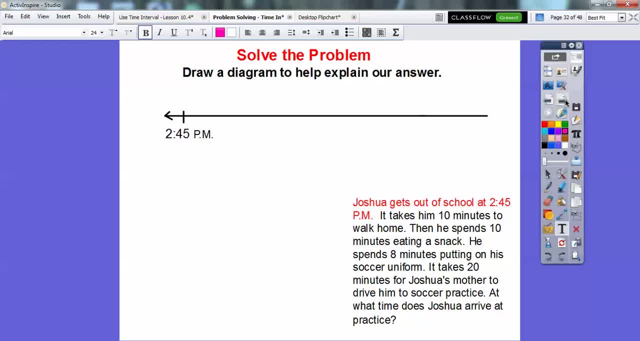 and we're going to jump forward on this. So let's draw a diagram to help explain our answer. So here's a number line right there. And so Joshua gets out of school at 2.45 pm. right there, okay. 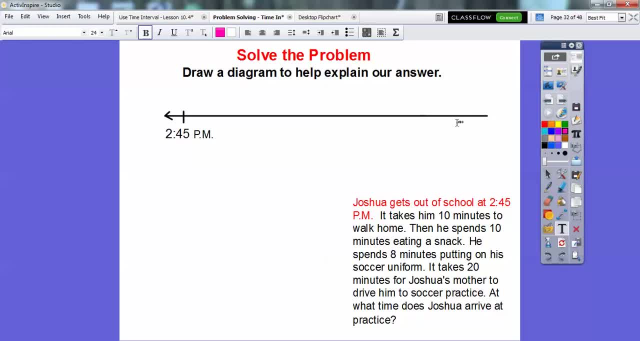 And so we're going to find out when he finally gets to soccer practice after we add all these minutes on. So here we go. It's going to take him 10 minutes to walk home. So that's here. it is in red right here. 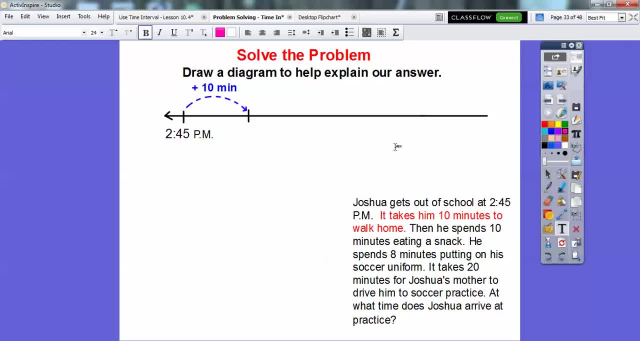 So let's add 10 minutes to 2.45.. That's going to take us to 2.55.. All right. this next sentence right here: it says he spends 10 minutes eating a snack. So we'll go ahead and add 10 minutes to that. 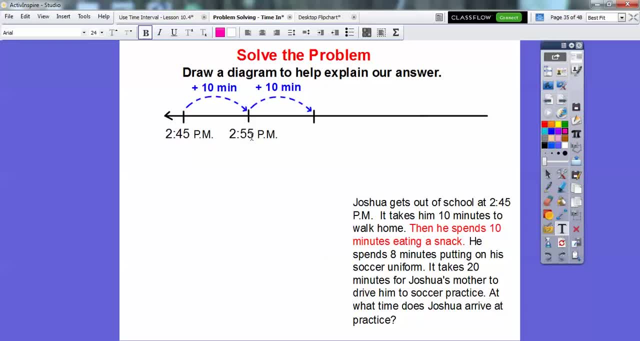 So 2.55 is right before 3 o'clock, So it's 5 minutes before 3 o'clock. So we want to add 10 minutes. So that's going to take us 5 minutes after 3 o'clock. That's going to be at 3.05.. 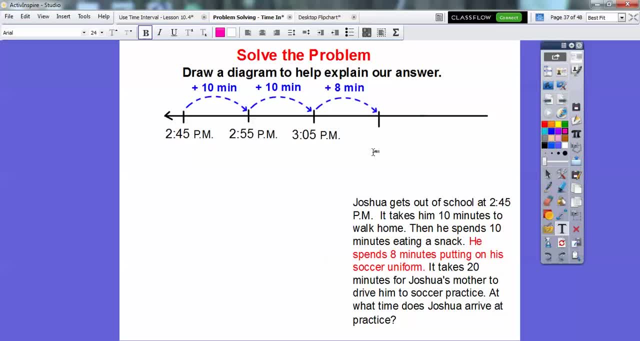 Okay, then he spends 8 minutes putting on his soccer uniform, So let's add 8 minutes to 3.05.. So use your fingers if you have to. So 3.05,, 3.06,, 7,, 8,, 9,, 10,, 11,, 12,, 13.. 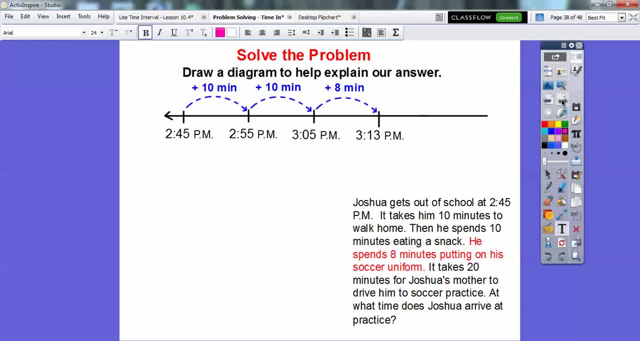 It's going to take us to 3.13.. I was using my fingers. Okay, that's okay. My students in high school use their fingers still all the time to count numbers. okay, I do too, All right. and then so the last one says it takes 20 minutes. 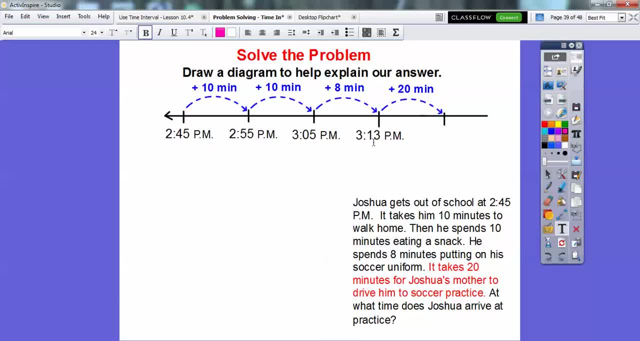 for Joshua to drive him to soccer practice. So if we add 20 minutes to this right here, so it's 3.13 plus 20.. It's going to take us to 3.33.. So let's go ahead and answer some questions here. 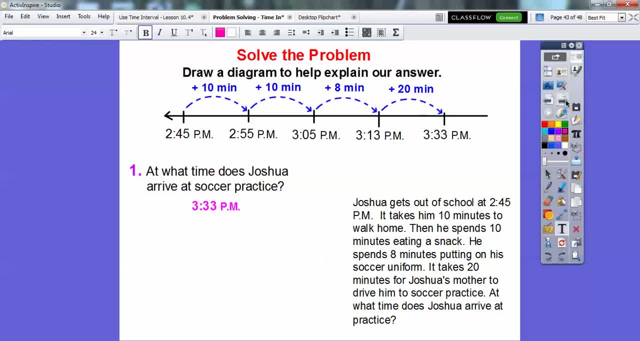 What time does Joshua arrive at soccer practice? Well, about 3.33.. So I don't know if his soccer practice is at 3.45 or, you know, 3.40 or whatever. So how do we know that this answer is reasonable? 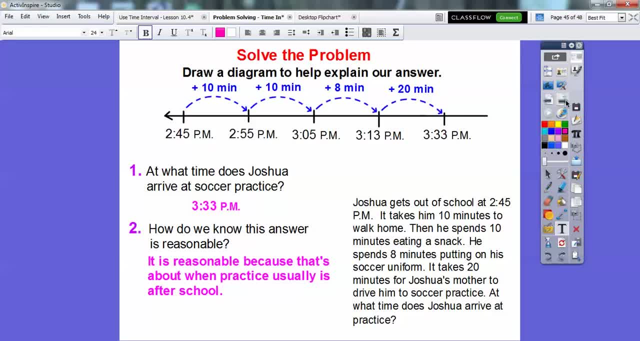 Well, if you have soccer practice or if you have a friend that has practice or baseball practice, it seems to be reasonable because that's when practice usually is, after school. So it's a little time to go home and change and eat a snack and all that stuff. 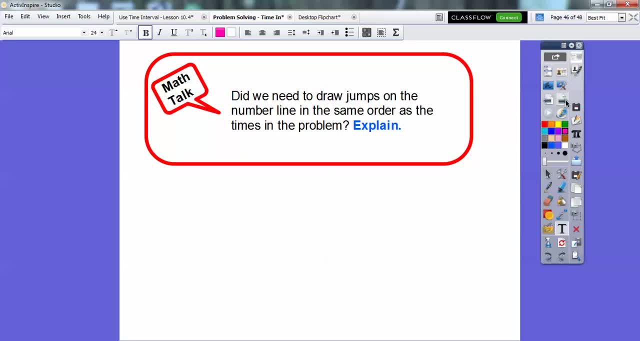 Okay, so did we have to draw those jumps on the number line in the same order as the times that were explained in the problem? Okay, well, no, because when we're adding all the numbers, it doesn't matter which numbers we add first. 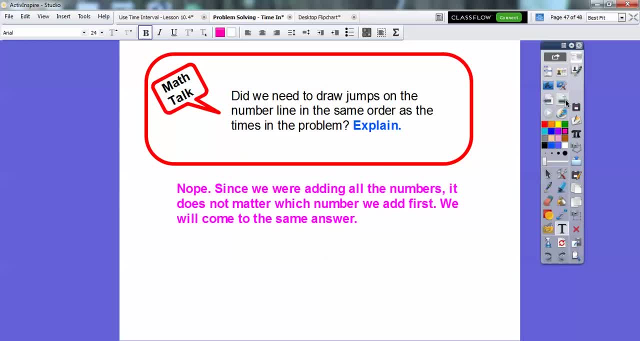 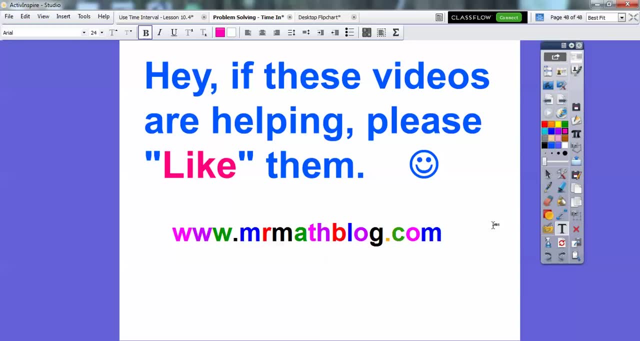 We're always going to come to the same answer, So we can add them in different orders if we wanted to, right there? Hey, if you're finding these videos helpful, would you please click Like. Thanks a lot, guys, Take care. Bye-bye. 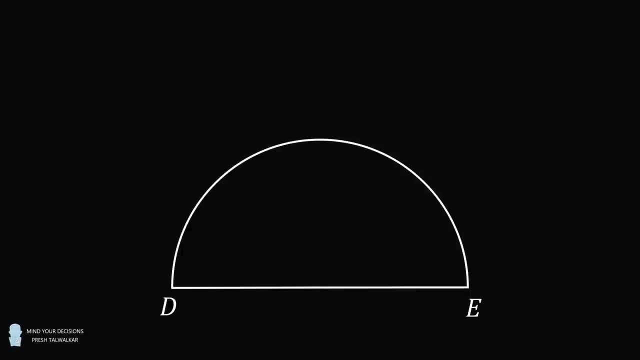 Hey, this is Presh Talwalkar. Semicircle DE has a right triangle DEF placed over it. where F is exterior to the semicircle, Let the region contained in the semicircle not contained in the triangle have an area equal to A and let the region exterior to the semicircle contained